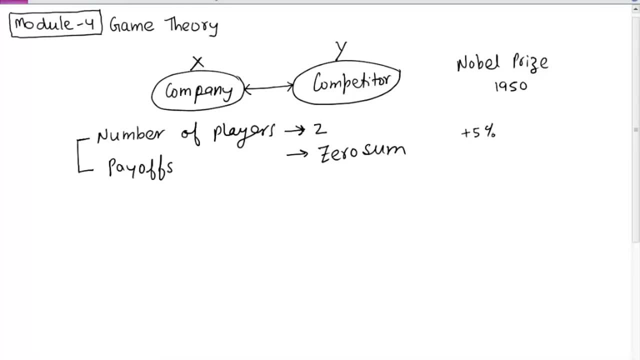 if there is a 5% gain for player x, that also means that there will be a loss of 5% for player y. so when you add these two, the total is always zero. so these type of situations are called zero sum games. another situation could be where player x chooses a strategy. 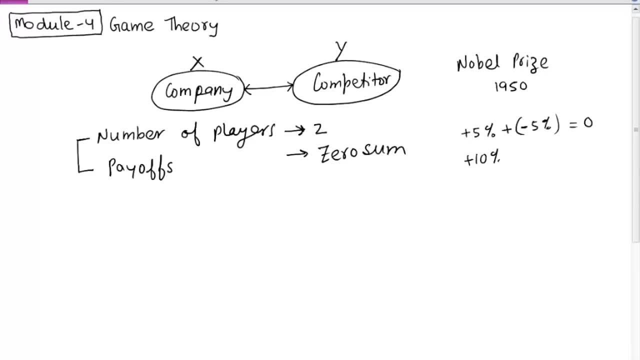 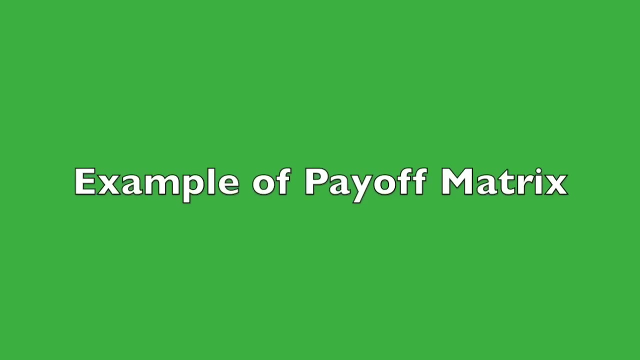 which leads to, let's say, 10% gain in the market share, and this gain is coming basically from the competitor who loses 10% market share. so the total is always zero. the third factor in game theory are number of strategies players can choose. let's consider situations where these two players, x and y, 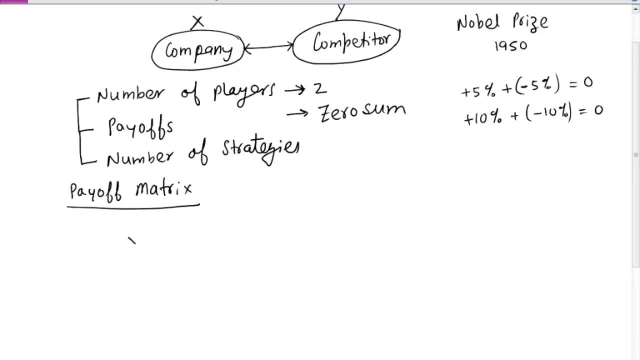 they choose two strategies. suppose x1 represents the first strategy by player x and x2 represents second strategy by player x. these two strategies could be, if we are looking at, say, marketing. maybe first strategy is using TV for ads and second strategy could be using radio for ads. 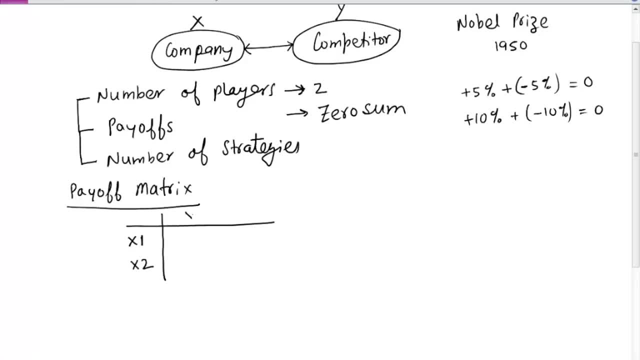 so, based on this, player y also will choose certain strategies and let's say there are two in this table. let's say payoff is three when x chooses strategy 1 and y chooses strategy 1. so this table is made with respect to player x. so if we see a positive number like 3, that means it is a gain for x and loss for y. 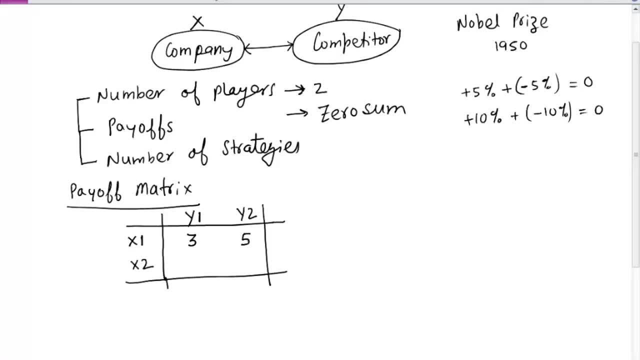 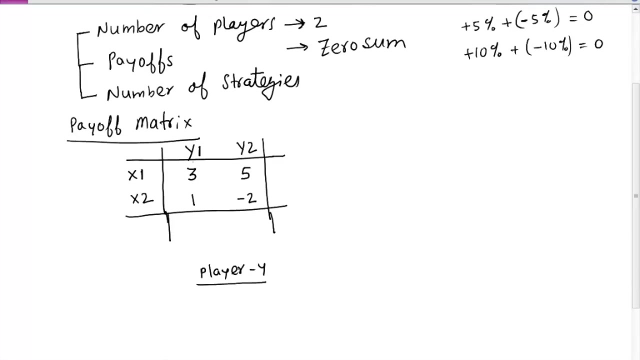 so let's say this value here is 5. so again it is gain for player x. this is 1. again this is discount, this is discount. so plus 3, that means it is a gain again for player x. this is negative 2, which means player x is going to lose. 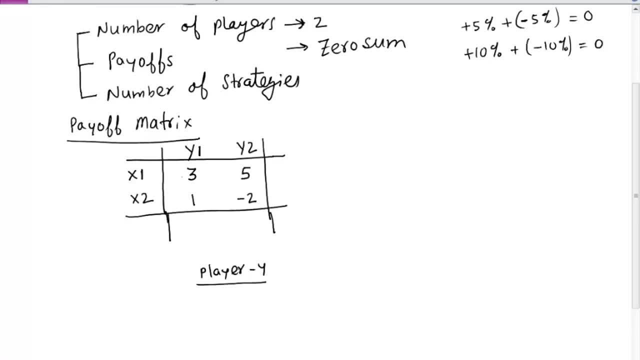 two points. so now, if you consider player y and the strategy is used by player y, when player y chooses 1st strategy, what will happen is: if x chooses 1st strategy, y will lose 3, and if player x chooses 2nd strategy, y will lose 1. 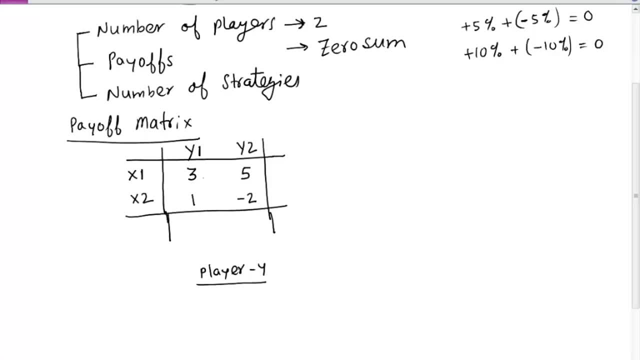 so maximum positive value of player x 1 is equal to negative into the negative number of pages x 1, so 3 and 2 by我. loss for player Y is going to be 3, so I am going to write maximum values in this last row. similarly, maximum possible loss for player Y will be 5 and basically. 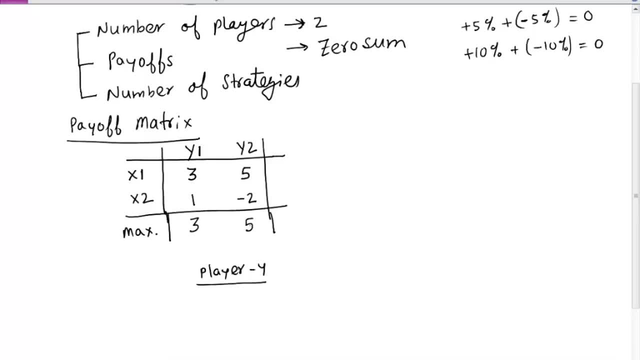 what player Y will try to do is to minimize the possible losses. so out of the two values, player Y will choose this one. and the idea is very simple, because this payoff matrix you can see out of four situation, three situations favor X, so obviously this payoff is biased towards player X, so Y is eventually. 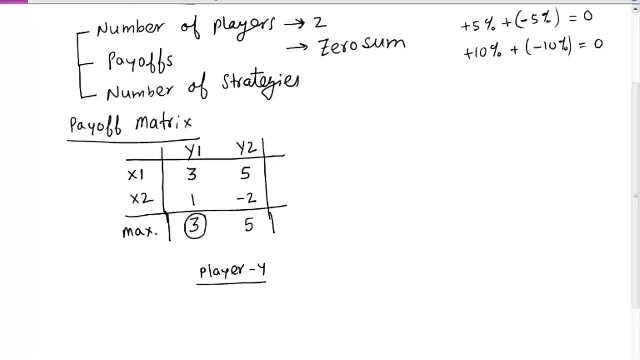 going to lose. the only thing Y can do is to minimize that maximum loss. the criteria being used by player Y in this situation is minimax criteria, which is minimizing the maximum loss. This three here is called upper value of the game. Similarly, if you consider strategies used by player X, So what player? 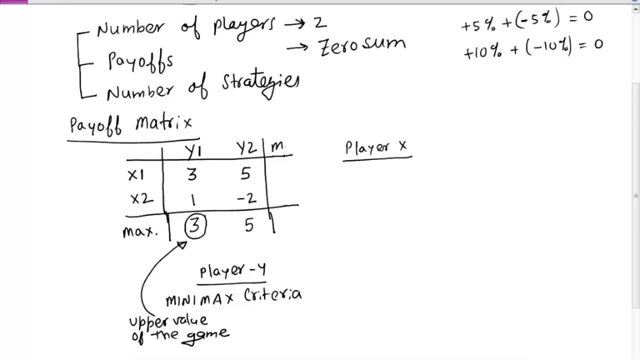 X will try to do is so if we create this last column where we put minimum payoffs, So in the first row minimum is 3.. So minimum possible win for player X using strategy 1 is 3.. Similarly, minimum possible gain by using strategy 2 is, in fact, negative 2.. So what? 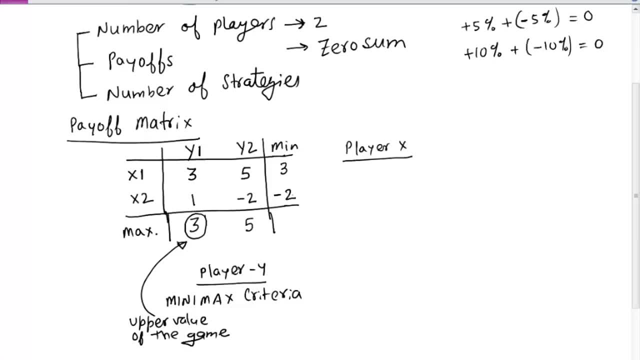 player X will try to do is player X will try to maximize the minimum win. So maximum of the 2 is 3.. This value 3 here, So player X is using a strategy called max win criteria And this value here is called lower value of the game. Now it happens in this case that the upper 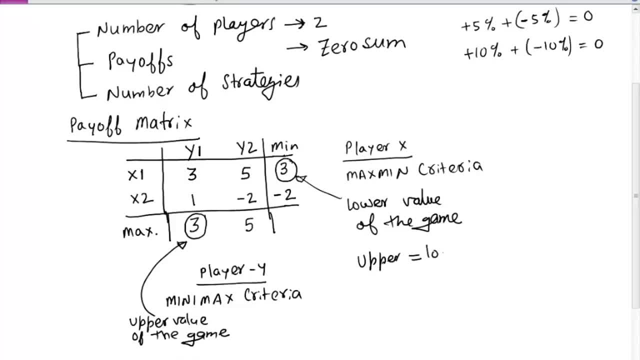 value of the game is equal to lower value of the game And in fact we can call this is the value of the game. So, basically, what is this number 3?? This number 3 is average or expected game outcome. if this game is played many times, like infinite number of times, So the game will converge. 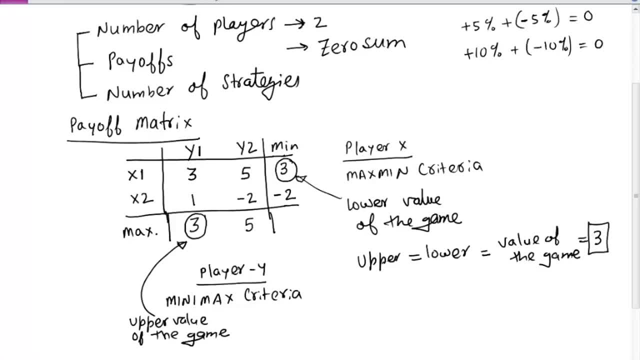 at this value 3.. So both player X and Y will use strategies in such a way that they end up with this value here. Basically it means, whenever player X chooses first strategy, Y will choose first strategy. Similarly, whenever Y chooses second strategy, obviously player 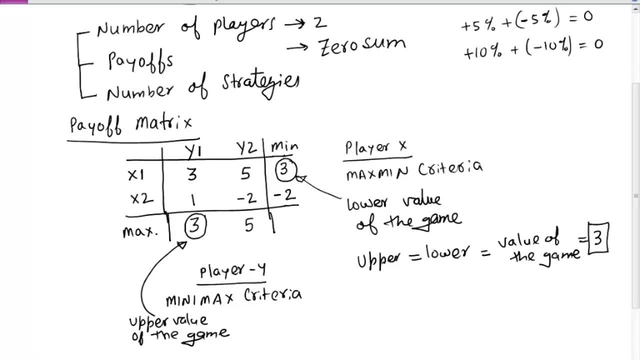 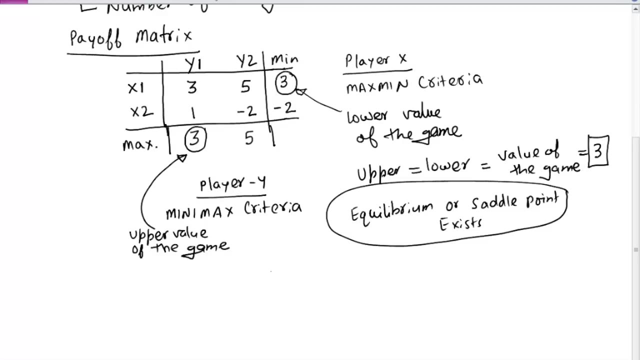 X will choose first strategy, So always they end up with 3.. So whenever this happens, whenever both these numbers are same, we say that equilibrium or saddle point exists. Equilibrium or saddle point exists, Equilibrium or saddle point. if we have this. so we have two situations. One is this point: 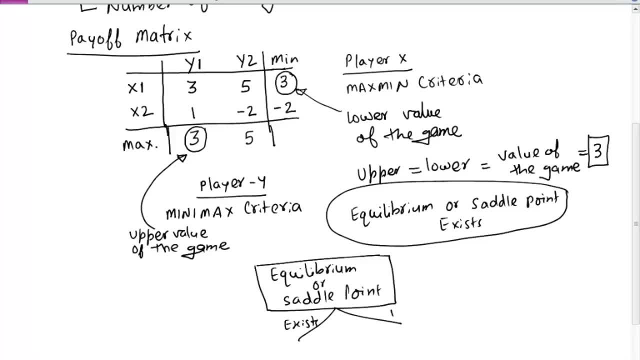 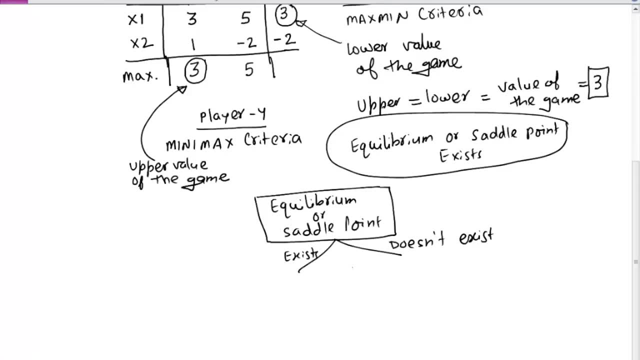 exists, and second situation is it does not exist. So whenever equilibrium or saddle point in a game exists, we say that we have pure strategy games, And when it does not exist, we say that we have pure strategy games. So pure strategy obviously means that both players will always use one particular strategy. 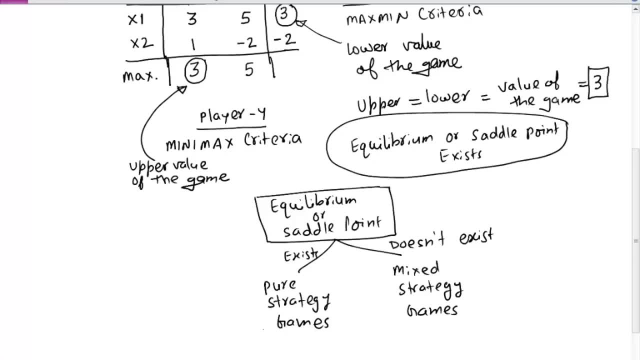 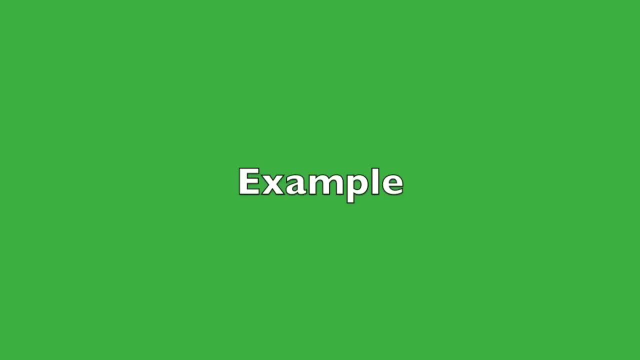 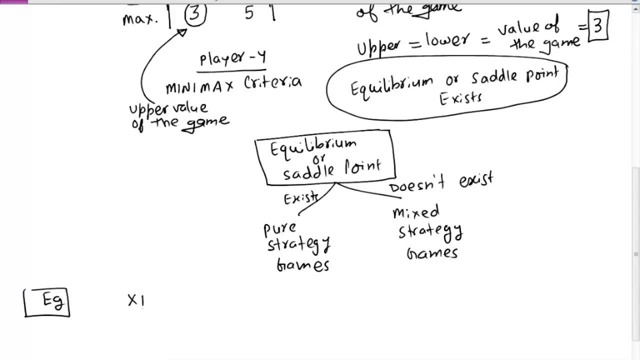 to maximize or optimize their situation. And mixed means. they may not use the same strategy all the time, They may change strategies. So let's say, payoff matrix looks like this: So suppose payoffs are 2, negative 4,, 6 and 10.. Now if you have to figure out whether 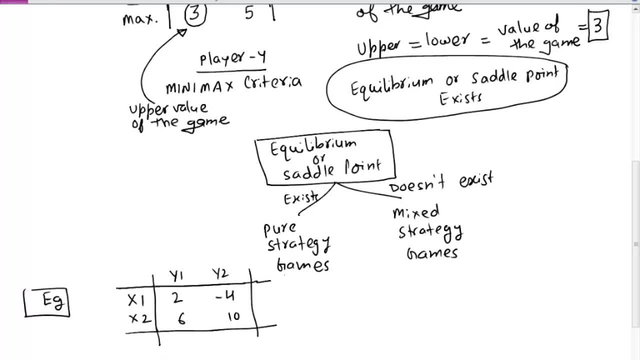 this is a pure strategy game or mixed strategy game. so we again apply Minimax criteria for player Y. So if we find maximum value in those columns, so maximum is 6 and 10.. So we select minimum of the two using minimax criteria. 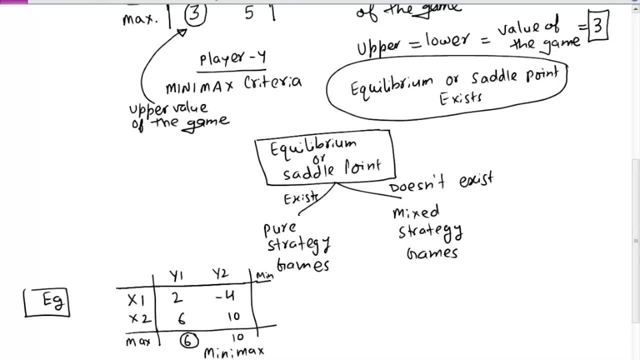 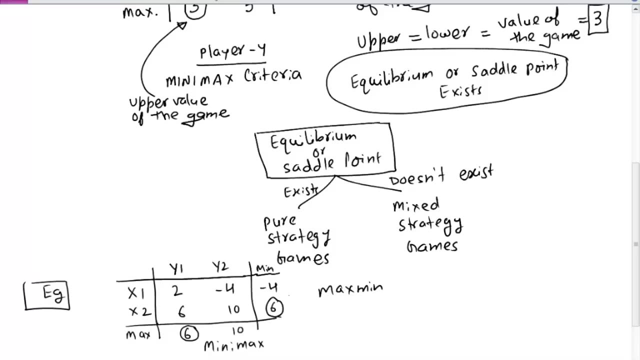 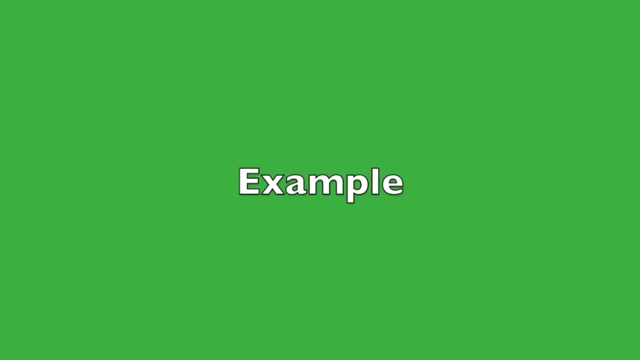 similarly, if you find minimum in the rows for player x, so negative 4 and 6. so if we use maximum criteria, so maximum of these minimum values, so the value is 6, so again both are equal. so this is also pure strategy game. so this previous example also, you can see it is 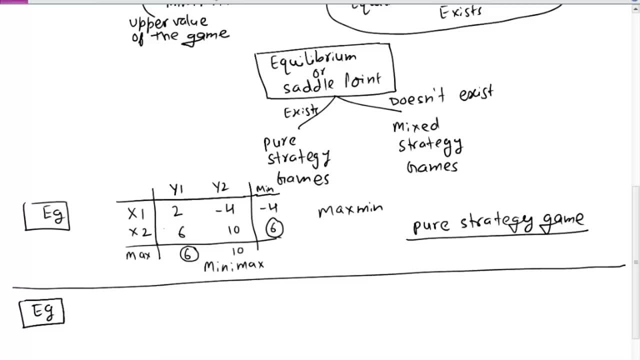 favoring player x because, out of four situations, in three situations it favors player x. so let's look at this one- x1, x2, y1 and y2- and suppose the payoffs are 10, 7, 6 negative 12 and 2. 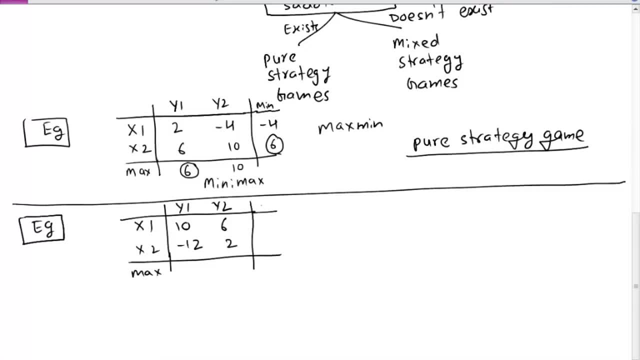 so again, if you find maximum and minimum values, so you have maximum 10 and maximum 6 here, and minimum of the two is 6 using minimax and similarly using maxmin, 6 negative 12, so maximum of the two is 6. so again we have: 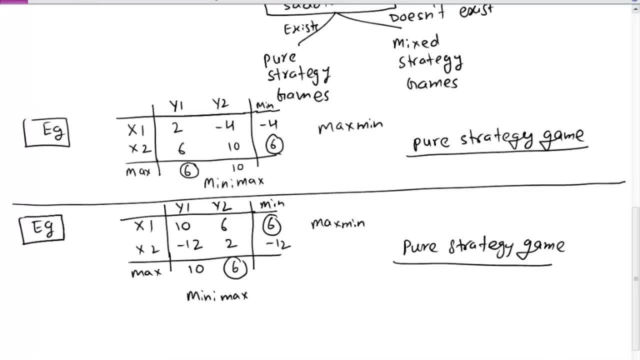 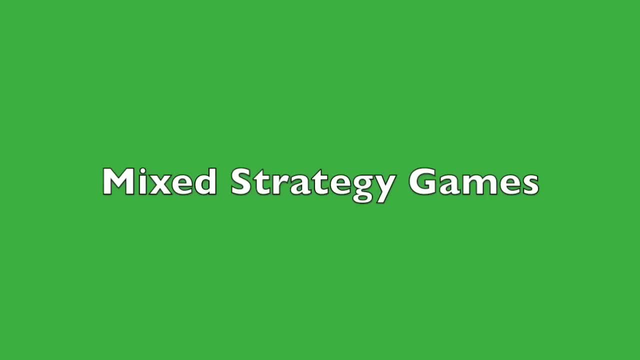 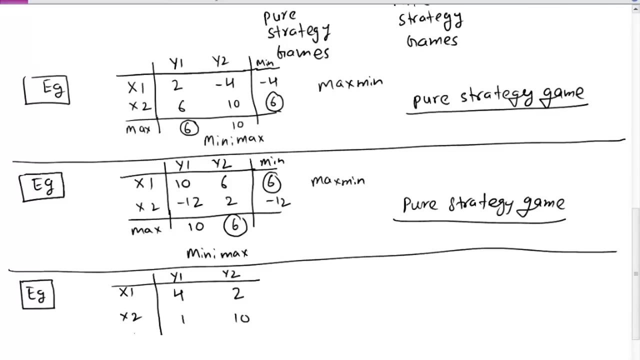 pure strategy game, so always only one solution will appear. so this game also favors player x, so maximum of the two is 2. so now they do not match. so obviously this is called mixed strategy campaign. so if you want to play it in a different way, this can also do that next time. 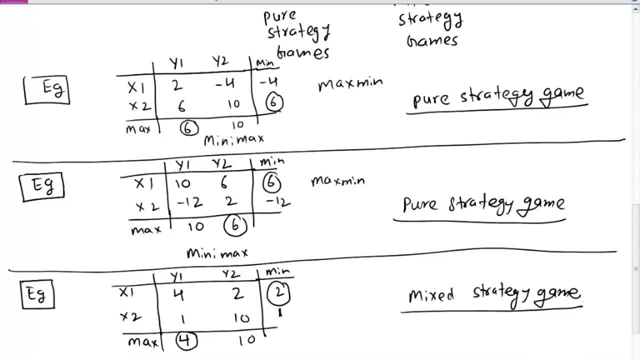 game, For big strategy game, to find the expected value, like if the game is played for a long period of time. so what is the expected gain for player X or what is the expected gain for player Y, To find that we have to do this analysis in slightly different way. It's not. 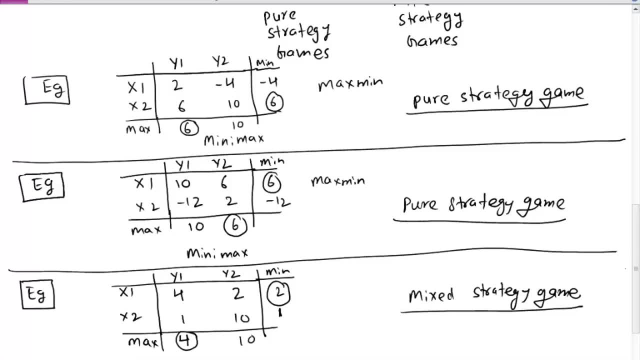 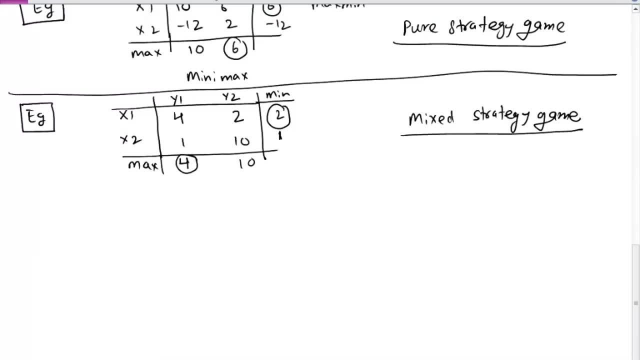 as straight forward as we have done in the previous examples. So we need to do some calculation to figure out what is the expected value for the two players. So I'm going to again make this table here slightly bigger so that I can write few other values. so 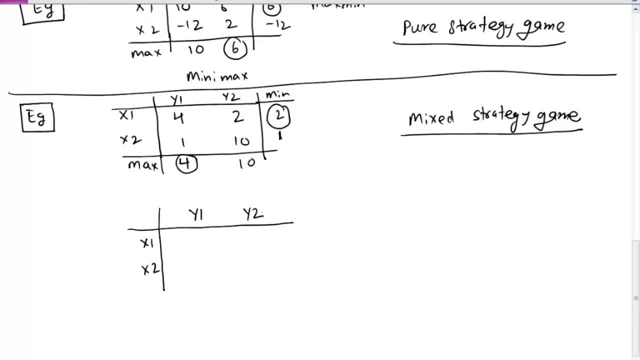 and let's say player Y plays strategy 1: p times and strategy 2 1 minus p. Proportion of times strategy 1 is played is p, and proportion of total times when strategy 2 is used by player Y is 1 minus p, so that the total is always 1. 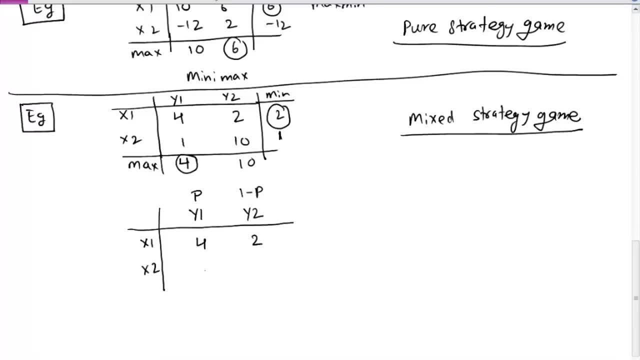 and p is 4, 2, 1, 10 and similarly for player X. let's say, first strategy is used q times, or proportion is q and 1 minus q for second one. So expected gain will be 4 times q. we multiply 4 in q, so basically: 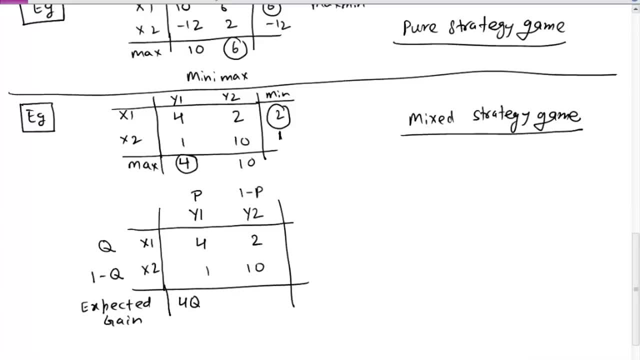 we are taking weighted average. We are using the weights as the proportion of times each payoff will occur. So 1 times 1 minus q. similarly, 2 times q for this, one plus ten times p times q for second one, 1 minus Q. So now, if we 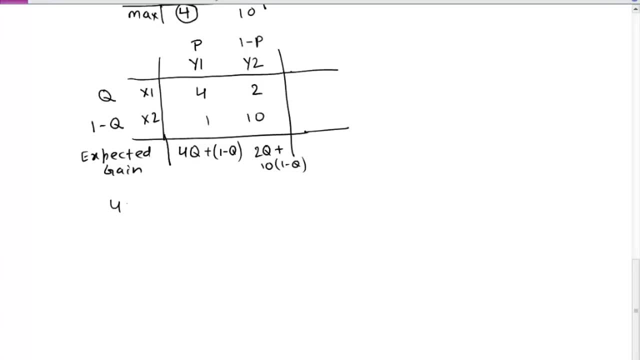 equate the two, what we are going to get here is 4Q plus 1 minus Q equals 2Q plus 10, 1 minus Q. Basically, we are trying to figure out what will be the value of QB. If you simplify this, you get: 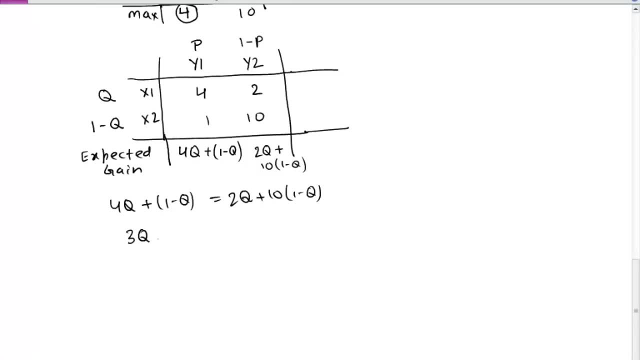 4Q minus Q is 3Q plus 1 and if you simplify this, you get negative 8Q plus 10.. So you end up with: if you bring negative 8Q this side, so you end up with: 3Q plus 8Q equals 10 minus 1.. 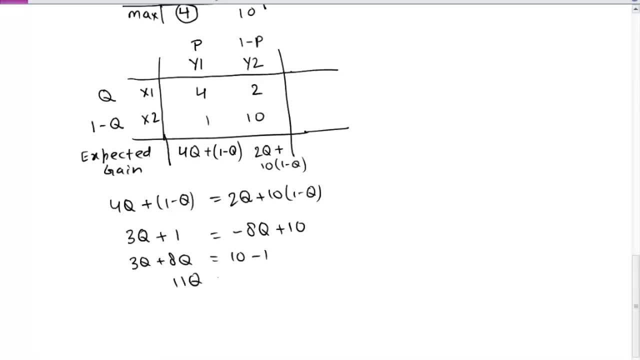 So in fact 11Q equals 9.. So your Q is equal to 9 over 11.. So if Q is 9 over 11, so obviously 1 minus Q is going to be 2 over 11.. So basically, player X will play first strategy. 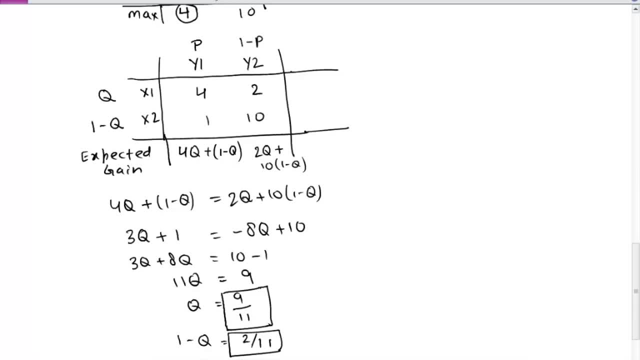 9 over 11, like that will be the proportion out of all the time player X will play. Player X will play strategy 1, and similarly 2 over 11 for strategy 2.. Now, similarly, if we calculate expected gain, so now we multiply 4 with P, 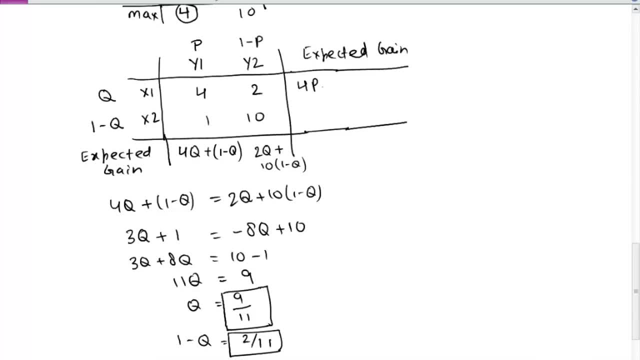 so 4P plus 2 times 1 minus P, and then 1 times P is P plus 10 times 1 minus P. So if you equate the 2, you get this. If you rearrange so, 4P minus 2P will be 2P. 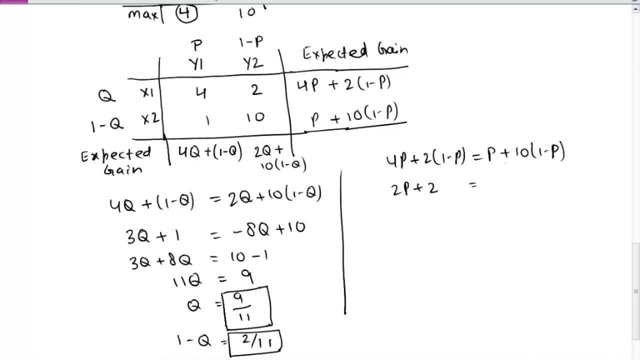 plus 2 equals, and this becomes 10 minus 9.. 9 plus 2 becomes 11 and this becomes 8, so that P equals 8 over 11.. Similarly, 1 minus P will be 3 over 11.. So, using this, if you want to calculate, 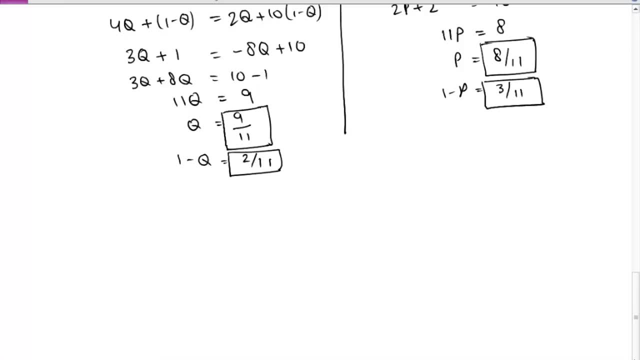 what will be the gain for, or expected gain for, Y? So you can actually use any one of the two. Let's say I'm using the second one. so P plus 10 times 1 minus P. So if you input these values here, 8 over 11. 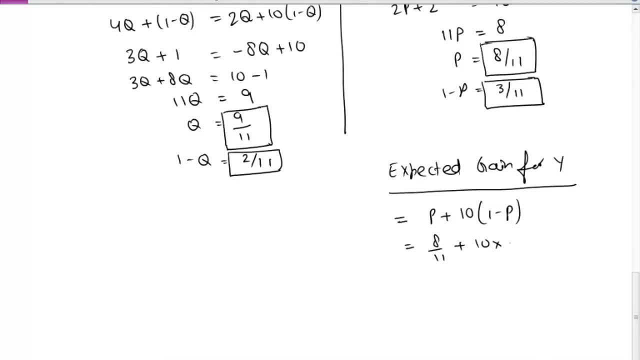 10 times, because 1 minus P is 3 over 11.. So 3 over 11.. So if you simplify this, you'll get 38 over 11, or 3.46.. Now expected gain for player Y: and because we are getting this 3.46, which? 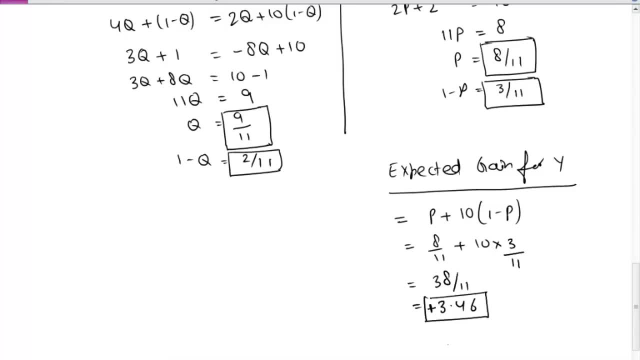 is a positive number. In fact, this is a loss for player Y because the payoff matrix is made in such a way that any positive value means it is loss for player Y and gain for player X. On an average, player Y is going to lose 3.6.. 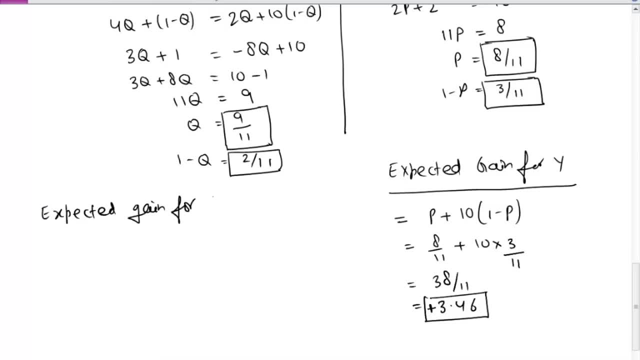 Expected gain for player X is going to be. So again, we can choose an equation. Let's choose the first one, This one here. This equals 4Q plus 1 minus Q. This becomes three times because Q is 9 over 11.. 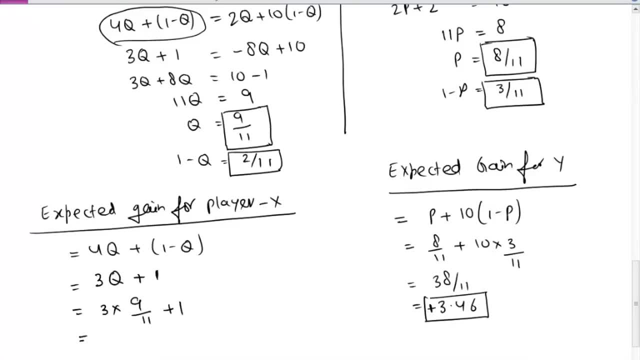 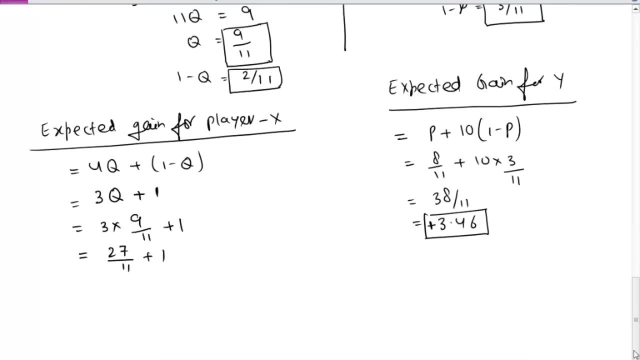 Plus 1.. So this will give us 27 over 11 plus 1.. If you simplify this, you get 38 over 11.. Which is same number we got earlier and we get 3.46.. These two numbers are obviously same because this is a zero. 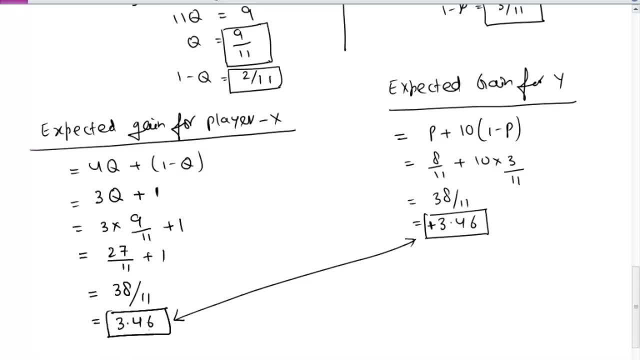 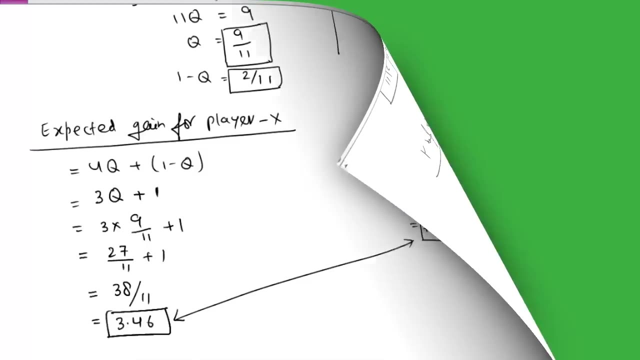 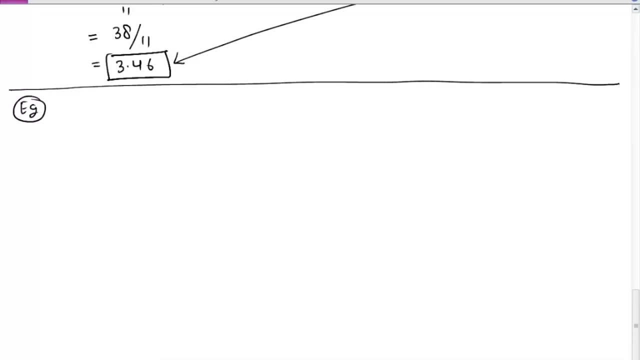 sum game. So whatever player X gains, same thing is lost by player Y, and whenever we see a positive number for player X, it means it is a gain, and if we see a positive number for player Y it is a loss. This time, let's say, this game favors. 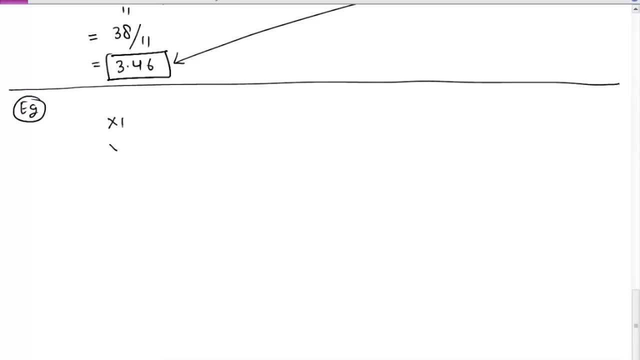 player Y, Payoff matrix is X1- X2.. So again, if you look at this and find using the max-min and min-max criteria, you will see that the two values of the game do not match. So this is also a mixed strategy game, So let's assume that. 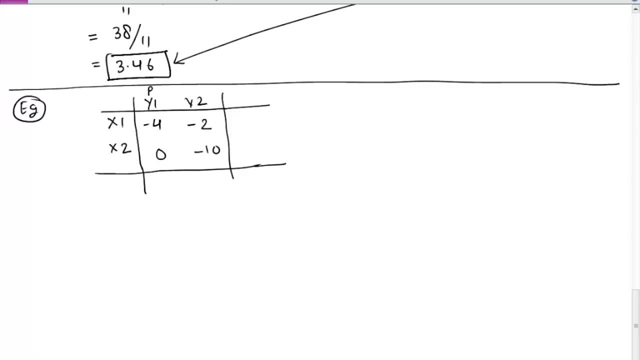 first strategy: by player Y is played P times and second strategy 1 minus P. That's the proportion and this is Q. So if you calculate this value here, negative 4Q and 0 times 1 minus Q is equal. We can equate with: 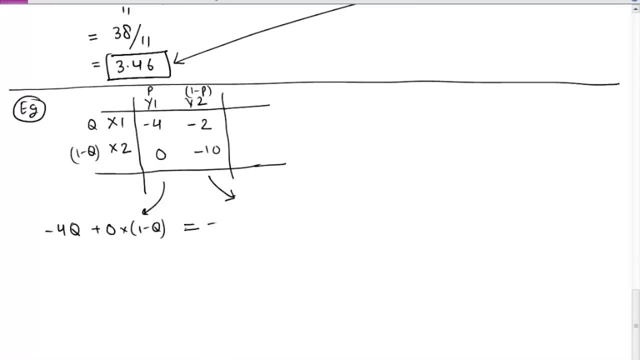 equal to the value here, which is negative 2Q plus negative 10 times 1 minus Q. So we are using these values here in the payoff table and multiplying by the proportions. So if you simplify this, this whole thing becomes 0.. So you're left. 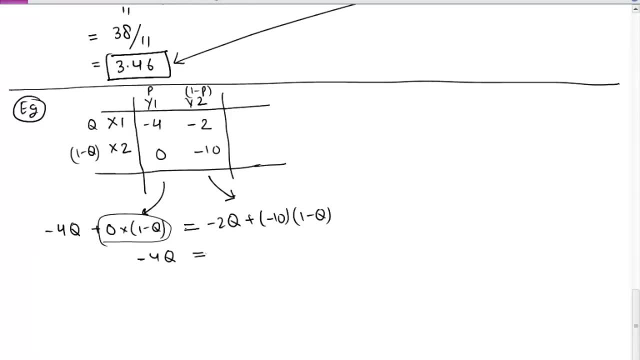 with negative 4Q and if you simplify this, you get negative 2Q, negative 10 plus 10Q. If you bring all the Q's on the other side, you will end up with negative 12Q and negative 10.. But 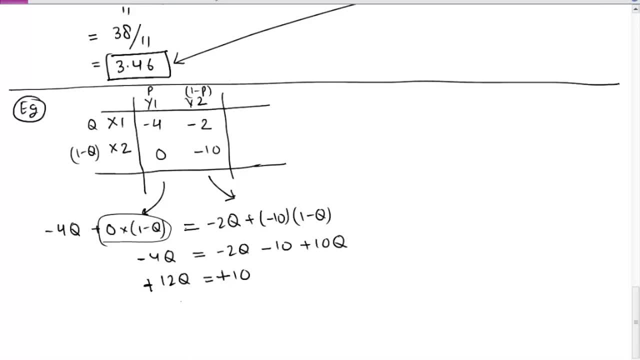 negative and negative become positive. So Q equals 10 by 12, which is same as 5 by 6.. So 1 minus Q obviously will be 1 by 6.. Now, if you do the calculation here, so this will be what we expected. 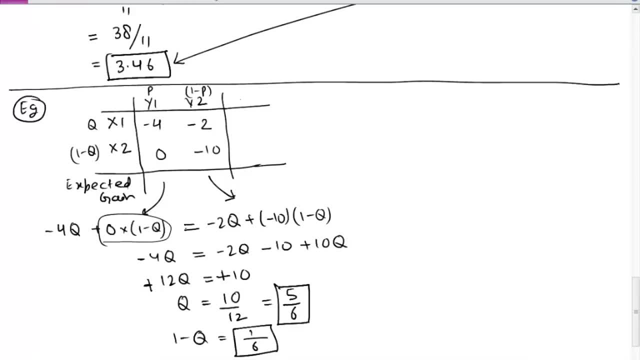 So if we equate the two, you get negative 4Q, negative 2, and this becomes plus. So 2Q equals So 0 times Q becomes 0. So you're left with negative 10 plus 10Q. 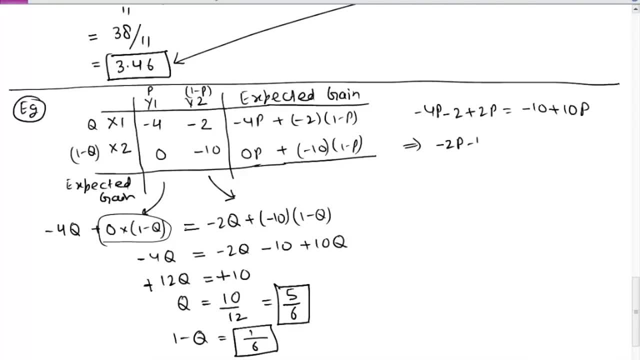 What you get here is negative. 2P minus 10P equals 2 minus 10.. If you bring all P's on the left and all the numbers on the right and then we end up with negative, 12P equals negative 8.. But because both 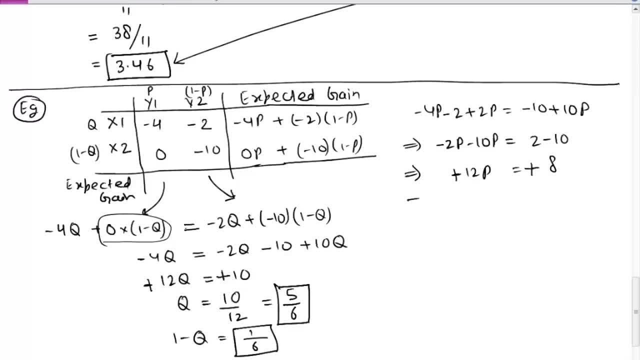 are negative so we can make it positive. So we get: P equals 8 by 12, or 4 times 2 is 8 and 4 times 3 is 12.. So 2 by 3. 1 minus P is going to be 1 by 3.. So based 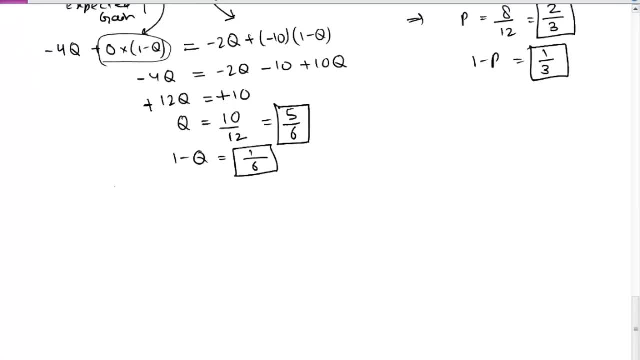 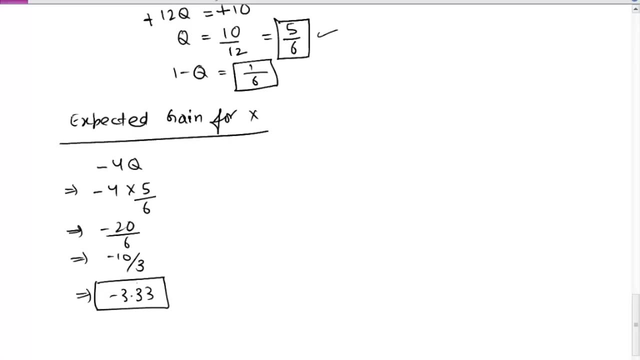 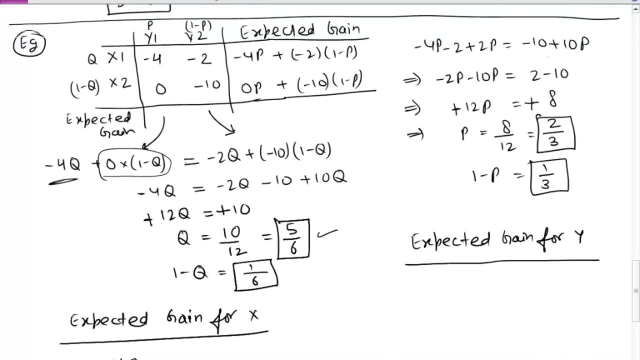 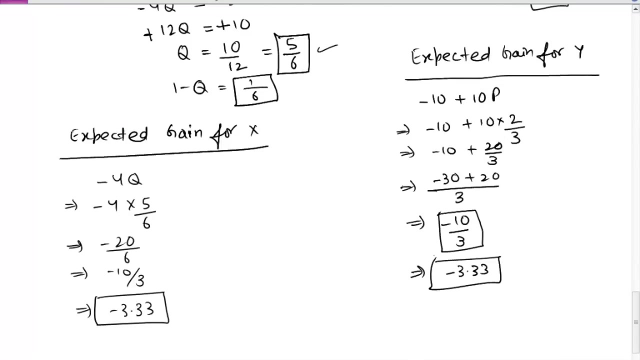 on the 2, we can calculate expected values. So negative value for player X means it is a loss for player X. So for player Y, if we see a negative number, that means actually it is a gain for player Y. You can see: both values are. 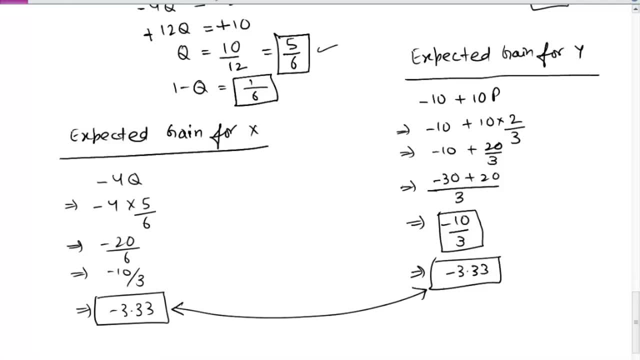 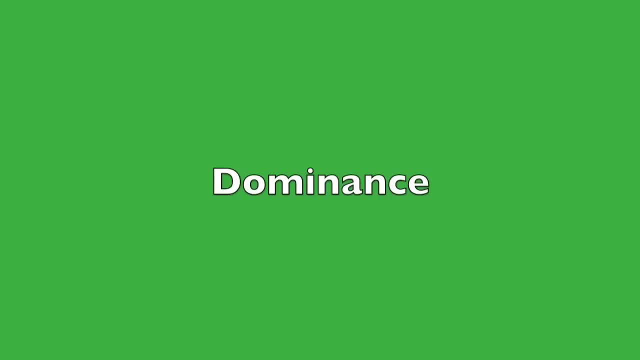 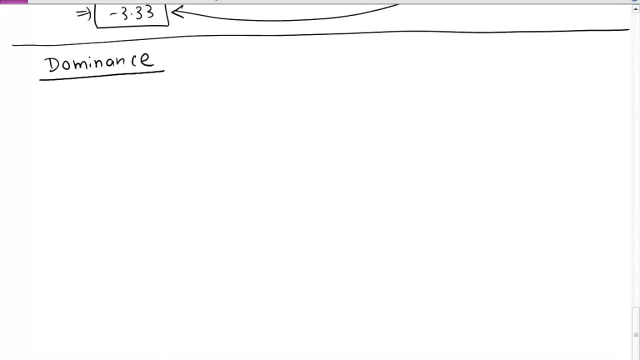 same but interpretation is different. So both are negative. So negative means loss for X but gain for Y. So the way this idea is used is: sometimes there are strategies which will never be used because the other strategies are so dominant that some strategies may not be. 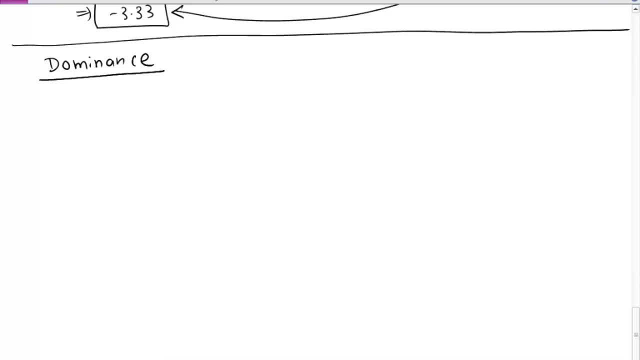 used anytime by any of the two players. When somebody is working to find a solution, it makes sense to eliminate those strategies which are dominated by other strategies, Because that will reduce the size of the game and make things more easier to do. So this is a very important point that we are going to discuss. 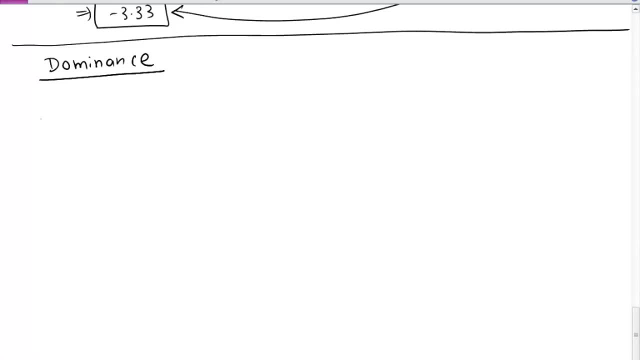 deal with. So let's say we have a situation like this- I will use example- where player X has X1, X2, X3, three strategies for the game and Y has two and, let's say, payoffs look like this: So when player X will use first strategy, obviously player Y will go for the. 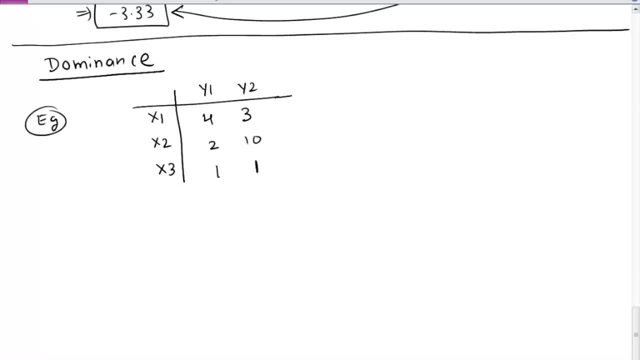 second strategy. When player X uses second strategy, player Y will go for the first strategy because that will minimize the loss. Now, in no case X is going to use the third strategy Because the payoffs are very small. In fact, player X will do better if player X goes for. 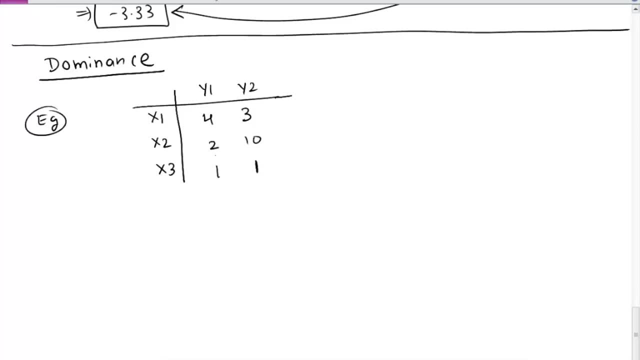 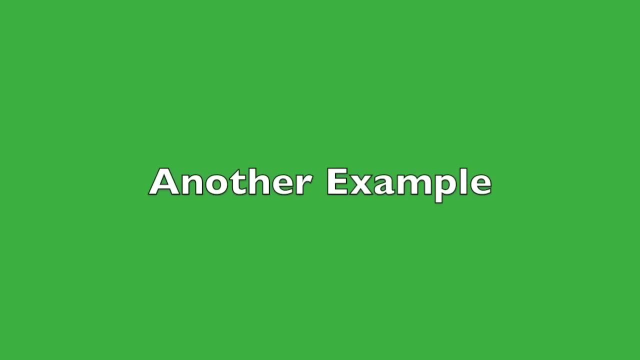 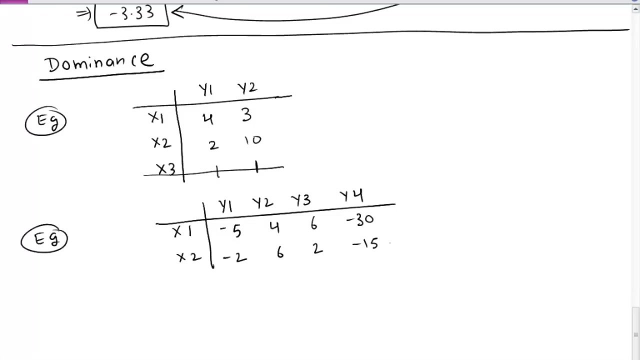 second strategy because the payoff will be at least two, which is two times. So this strategy will never be used because other strategies dominate this. So basically, this can be deleted. So if you look carefully at this payoff table, you will find that player Y will never choose.